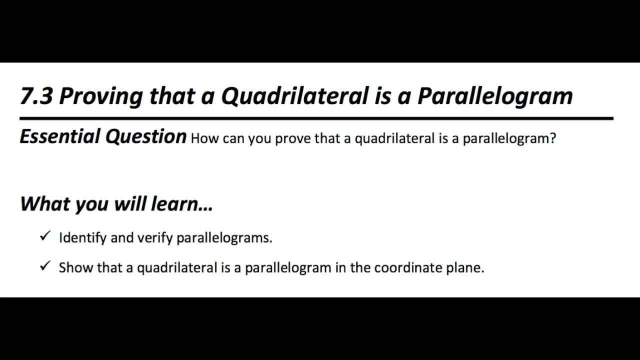 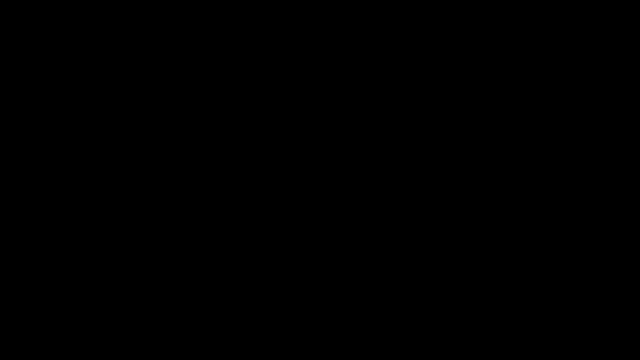 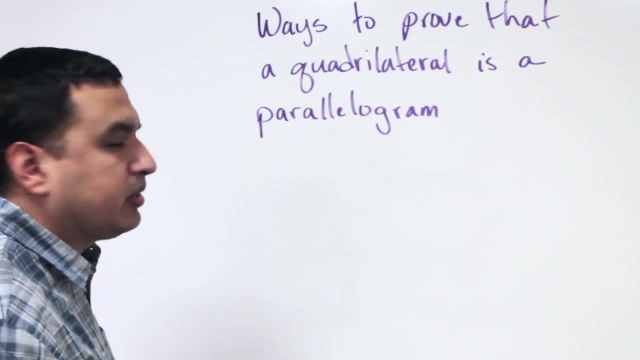 And we also want to show that a quadrilateral is a parallelogram in the coordinate plane. Okay, so today we're talking about different ways to show or to prove that a quadrilateral is a parallelogram. The first one I'm going to show you is actually just the definition of a parallelogram. 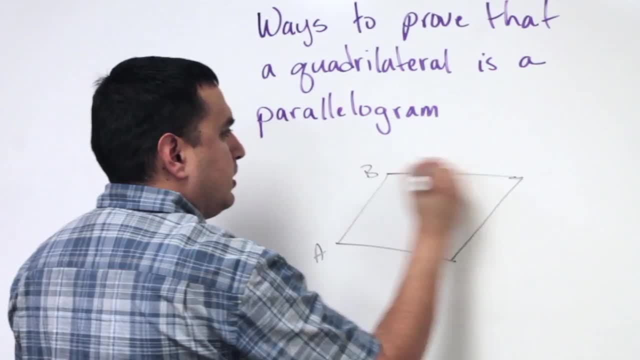 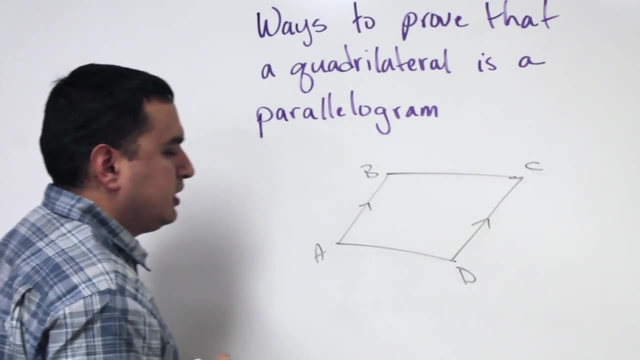 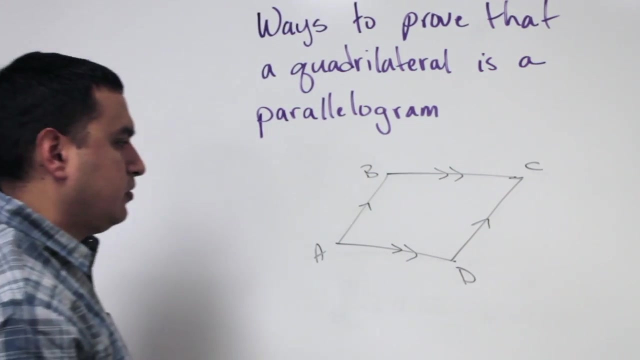 So if you're given some kind of quadrilateral ABCD and you can show that segment AB is parallel to segment CD and that segment BC is parallel to segment AD, then you can prove that you have a quadrilateral or you know that you have a quadrilateral. 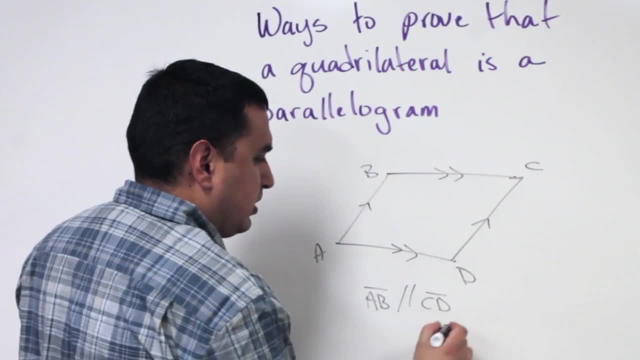 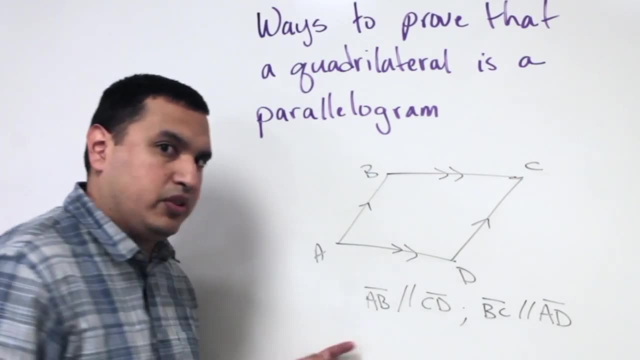 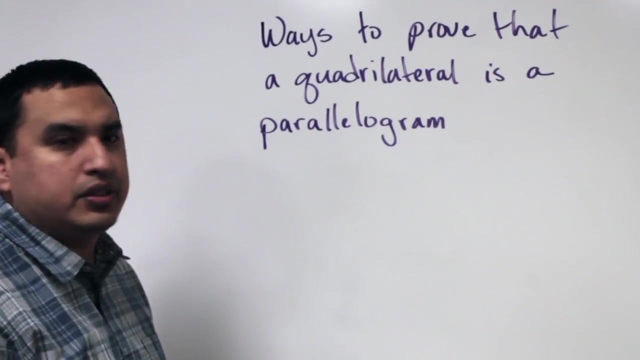 Let me just write it out: Segment AB is parallel to segment CD And segment BC is parallel to segment AD. Okay, if you can show these two statements, that means you have a parallelogram. Alright. the second way that we can do this is: 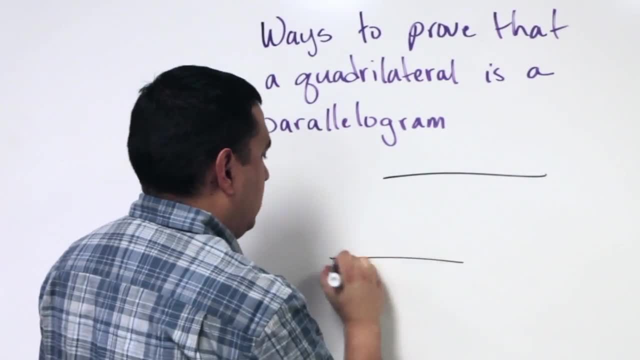 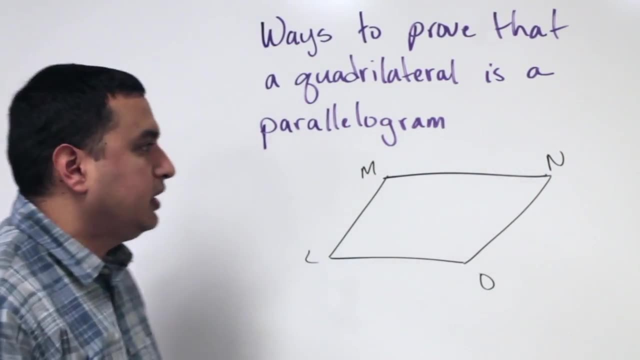 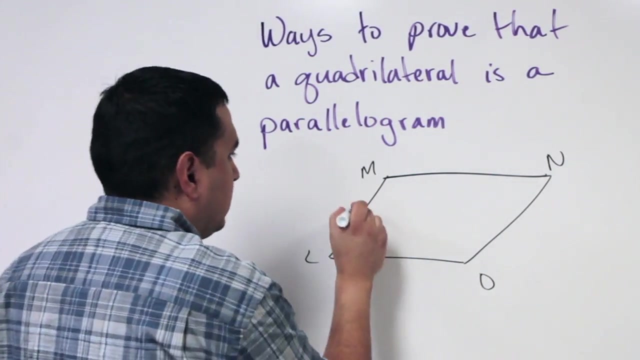 if we have some quadrilateral and let's just call this one- I don't know, L, M, N, O, and I know that, or I can prove somehow, either by something that's given to me or some way that I can figure out, that say, the segment L, M is congruent to segment N O. 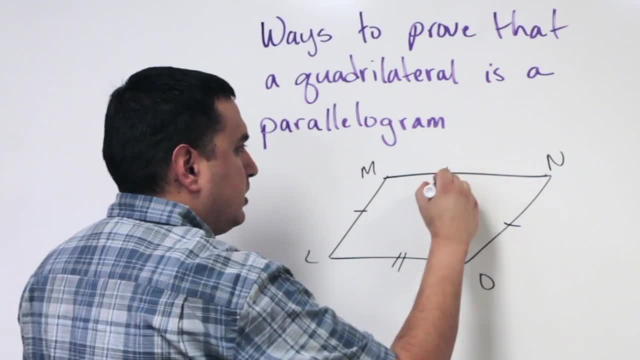 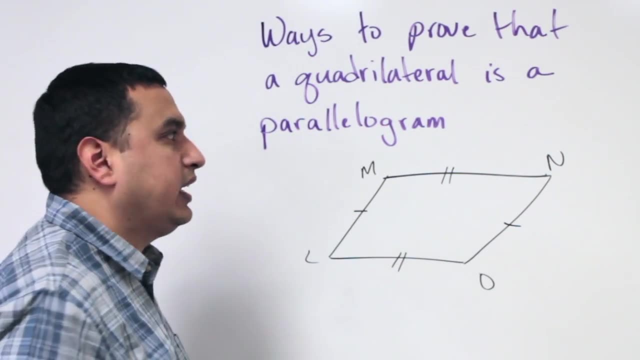 or O, N, and segment L, O is congruent to segment M- M. if I can prove those pair of opposite sides being congruent, then I know that I have a parallelogram. Okay, the third one, the third way that we're going to show. 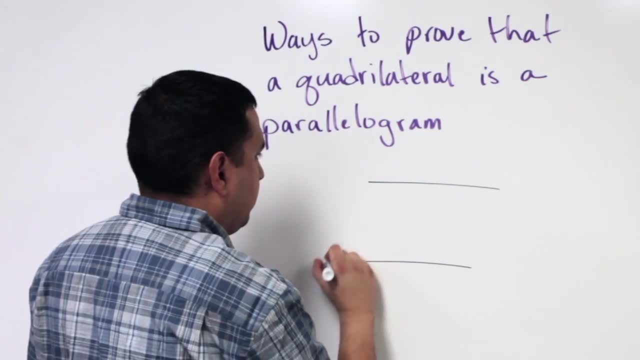 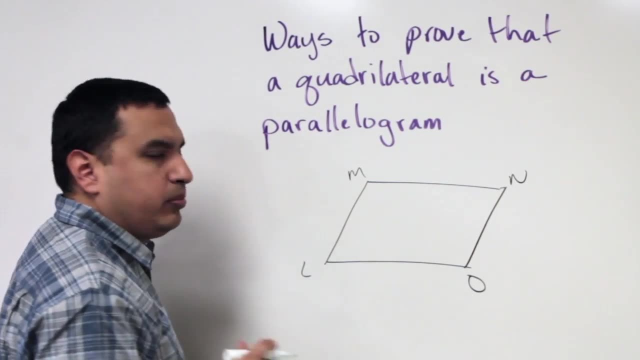 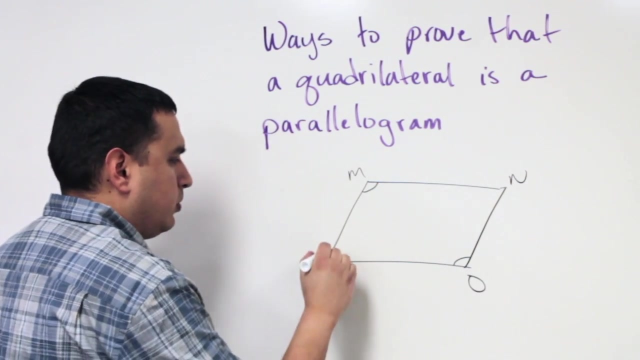 or prove that a quadrilateral is a parallelogram, is if, is if I can show that I have two pairs of opposite congruent angles, So somehow I can show that angle M is congruent to angle O, angle L is congruent to angle N. 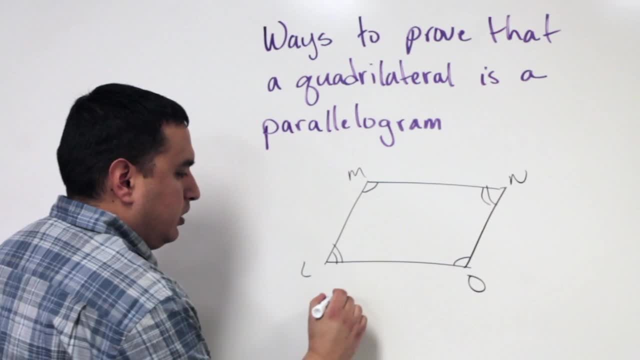 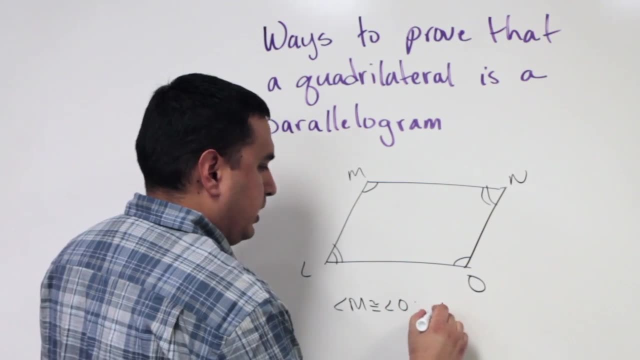 then I know that I have a parallelogram. Alright, so if you're writing these down, segment M is congruent to- or, excuse me, angle M congruent to angle O, and you have to show that angle L is congruent to angle N. 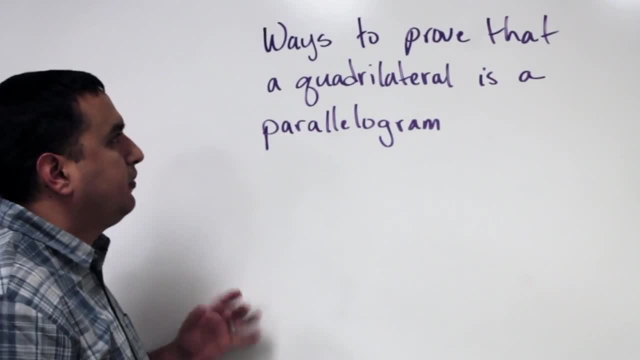 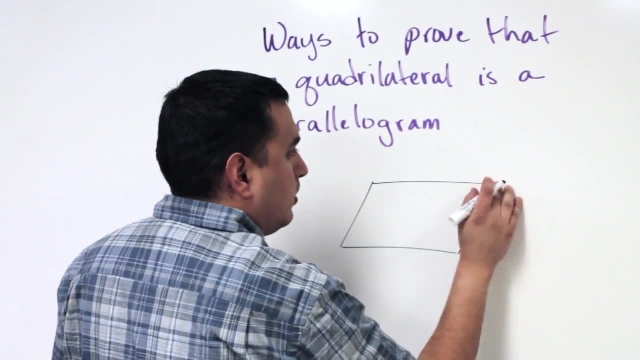 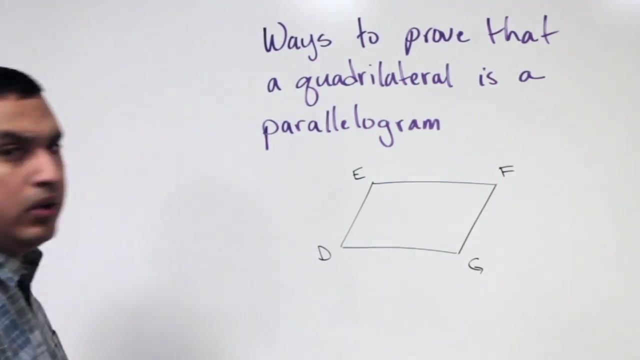 Opposite angles have to be congruent. Alright, the fourth way that we have, that we can show that a quadrilateral is a parallelogram. if we have some quadrilateral, Alright, we'll just call this one D, E, F, G and what I want to be able to prove. 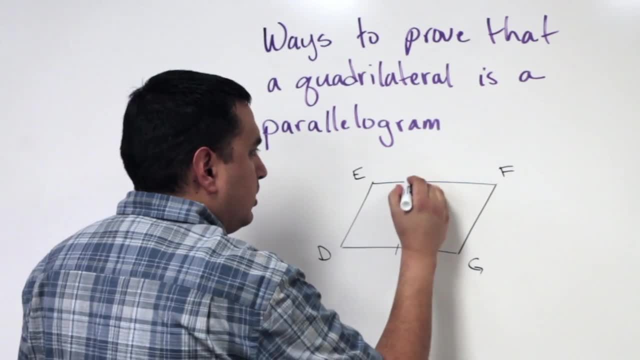 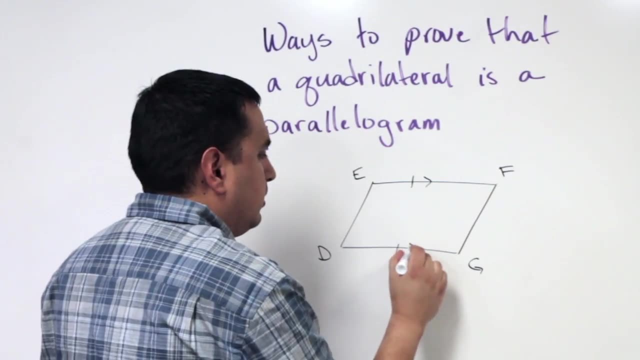 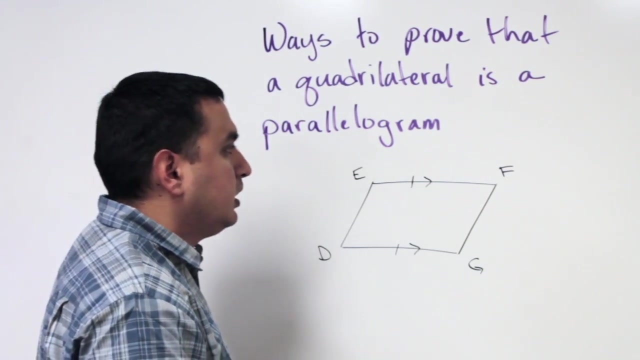 is that I have a pair of opposite congruent sides and also that those two sides are parallel. The other things that we talked about is I had to show two pairs of opposite sides being congruent and two pairs of opposite sides being parallel. This method just shows us that. 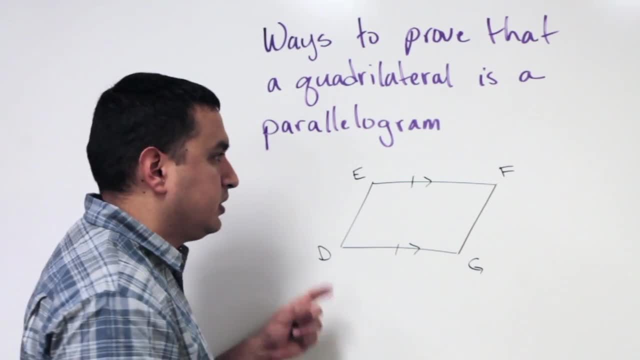 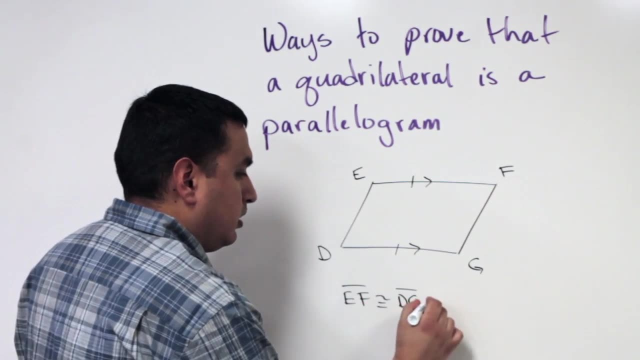 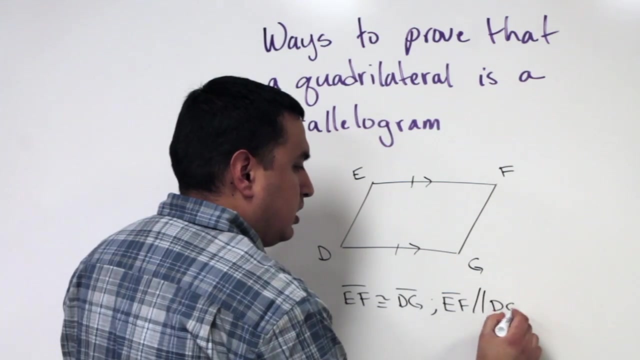 I only need to know one pair of sides that are congruent and also parallel. So if I can show E F, segment E F is congruent to segment D G and I can show that segment D G or segment E F is parallel to segment D G. 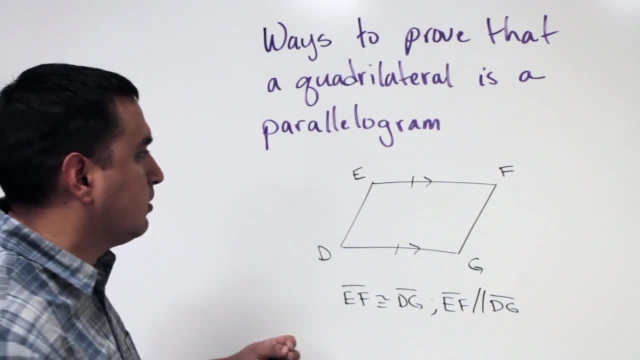 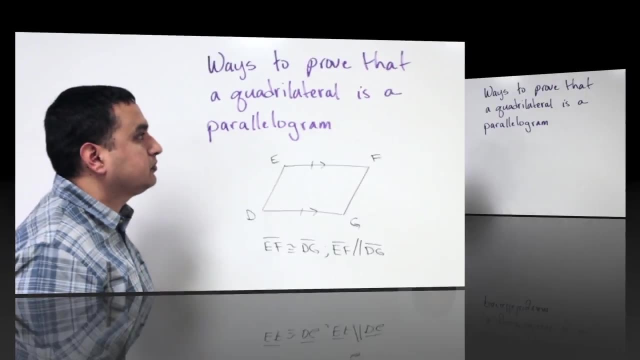 then I know the parallelogram or the quadrilateral is a parallelogram, And I don't have to know anything about segment D, E and segment G, F. Alright, the last method that we're going to talk about, or I'm going to show you today: 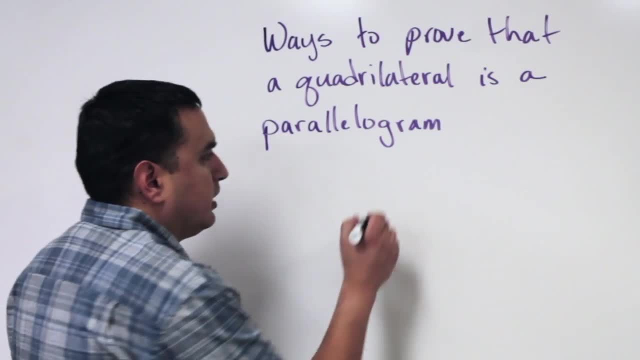 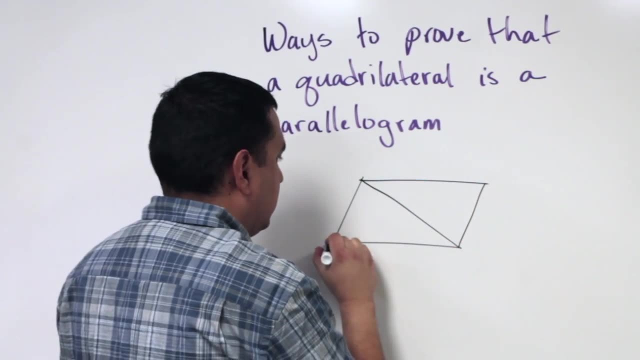 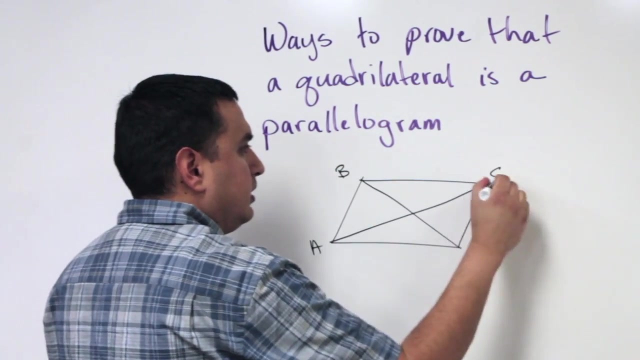 on how to prove that a quadrilateral is a parallelogram is: if I have some quadrilateral and I know that the diagonals bisect each other, then I have a parallelogram. So if let's go back to A, B, C, D, 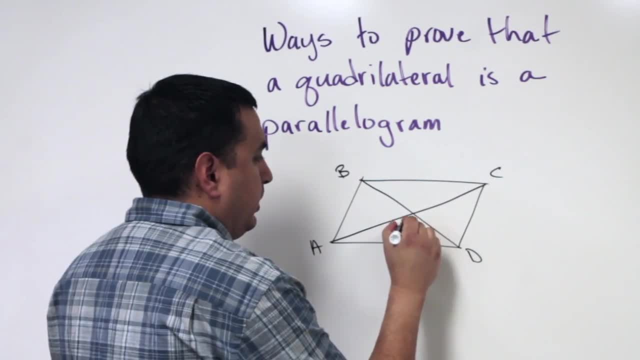 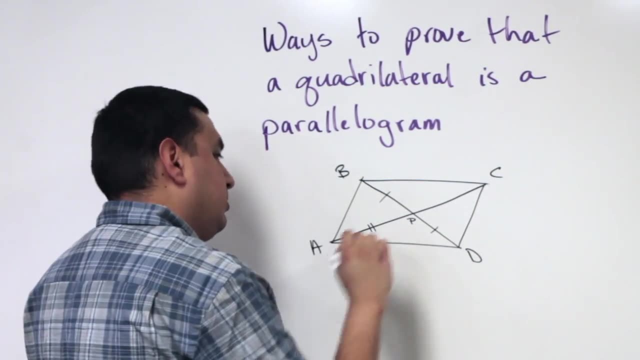 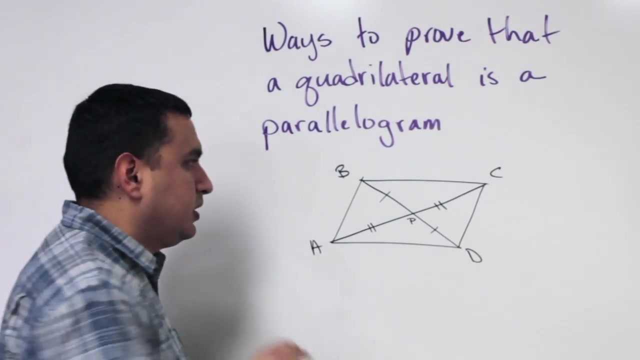 and we call this point P, I guess. and if I know that segment B P is congruent to segment D P and I can say that segment A P is congruent to segment C P, then that tells me that I have a parallelogram. I don't need to know anything about these outside parts. 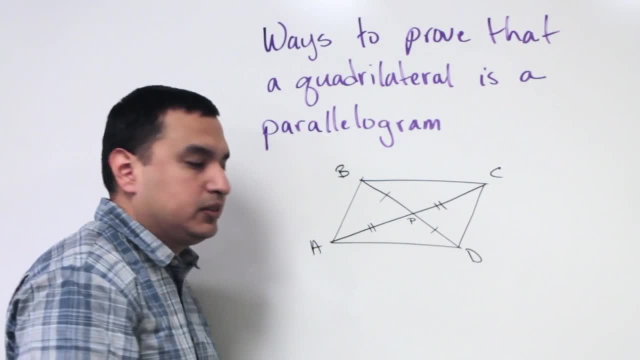 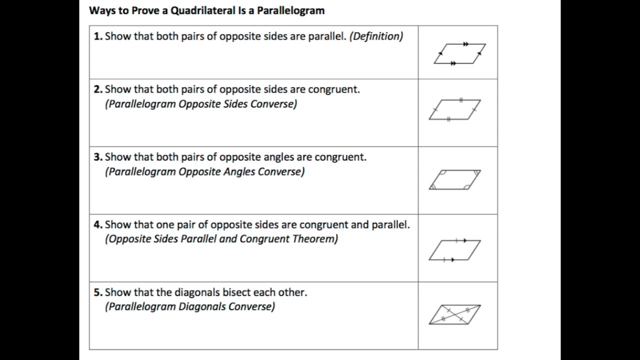 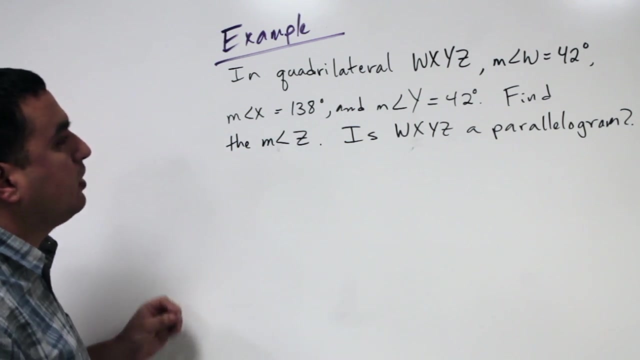 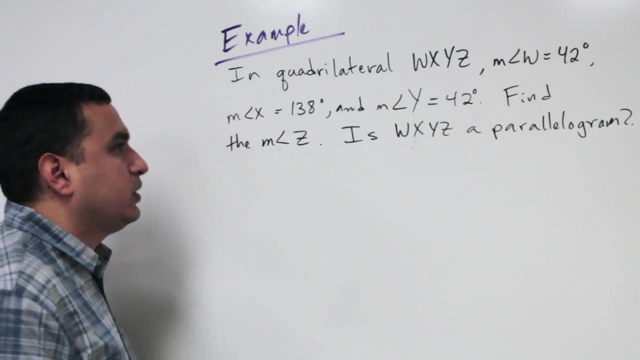 but I have to show that the diagonals bisect each other. Okay, this example: in quadrilateral W, X, Y, Z, the measure of angle W is 42, the measure of angle X is 138 and the measure of angle Y is 42. we want to find the measure of angle Z. 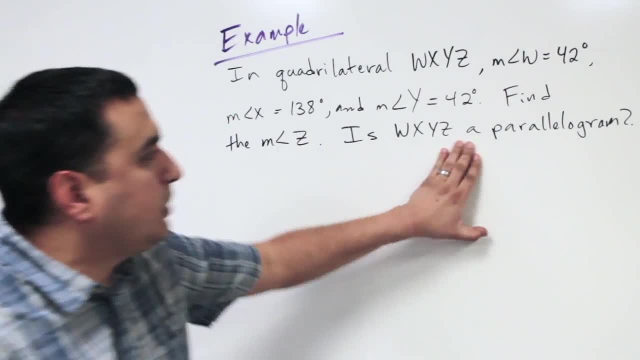 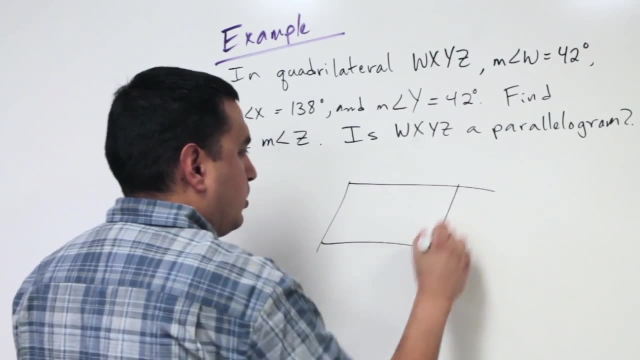 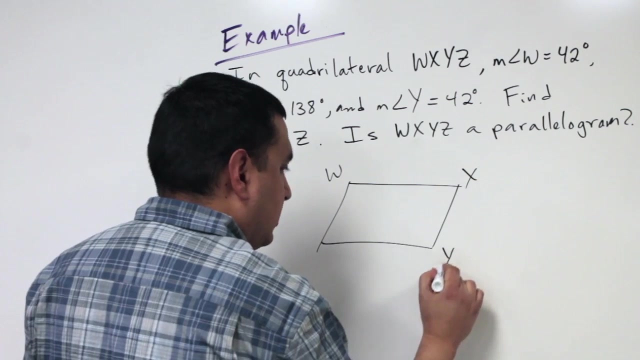 and we also want to ask the question: is W X, Y, Z, a parallelogram? Alright, so we want to start by drawing some shape or quadrilateral, not just a shape, and we're going to go ahead and call this W X, Y and Z. 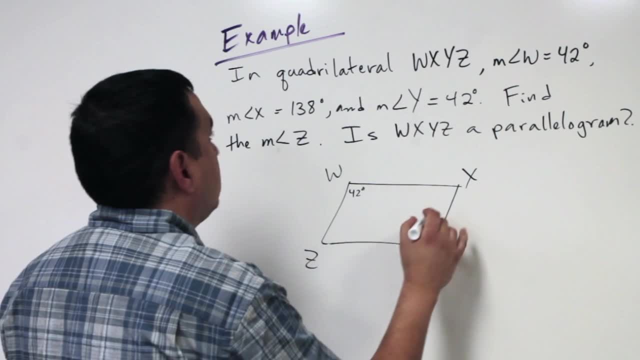 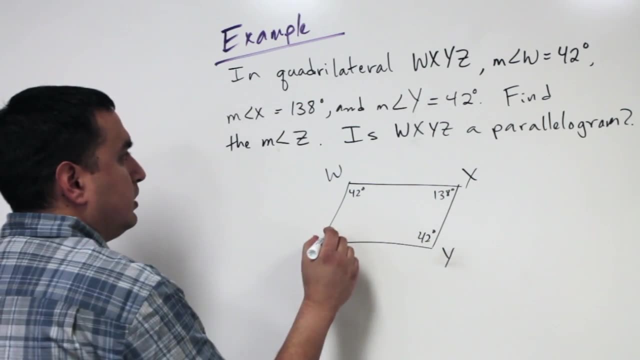 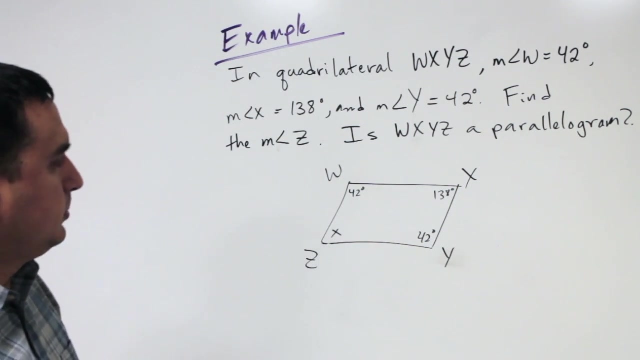 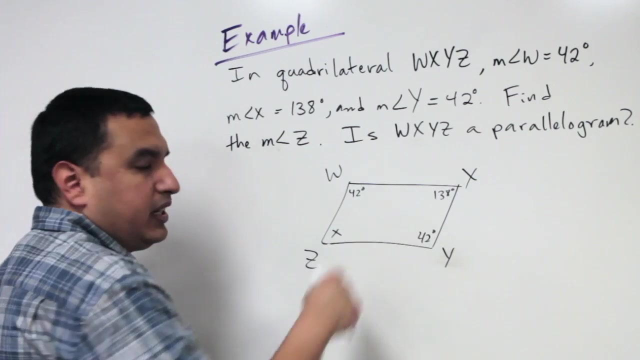 and I know that W is 42 degrees, X is 138, and then we have some unknown angle here. okay, so we have to figure out what that angle is, because it is a quadrilateral, I know all of these angles here have to add up to 360. 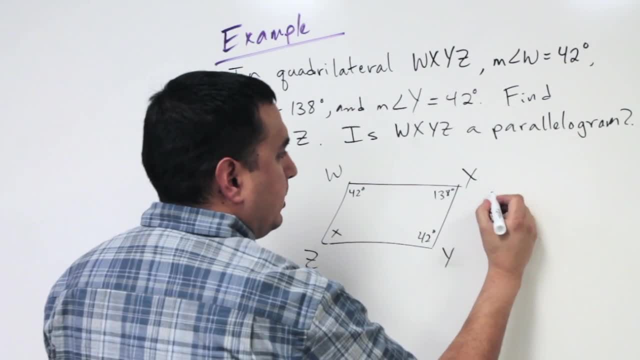 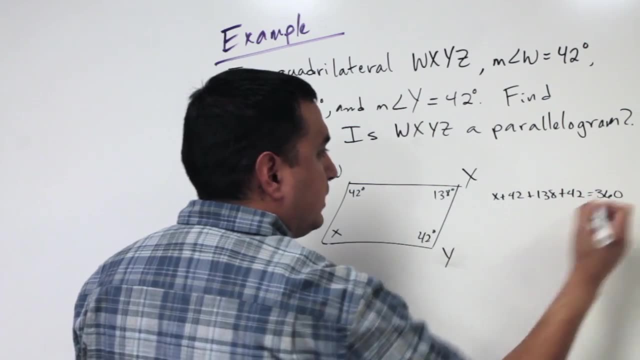 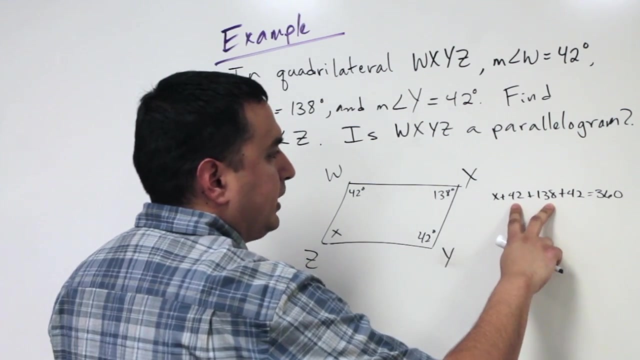 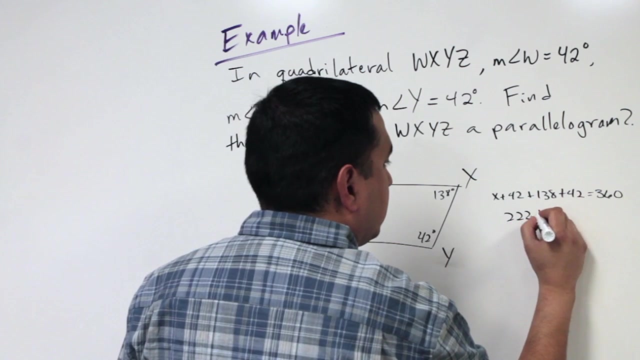 so if I take X plus 42 plus 138 plus 42 and set that equal to 360, I can solve that. let's see that's going to come out to be 180 plus 42 is going to be 222. so 222 plus X. 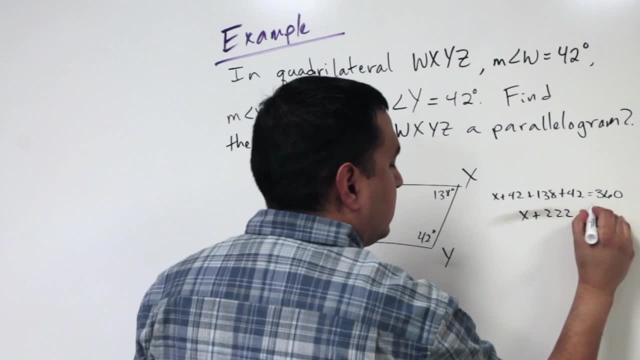 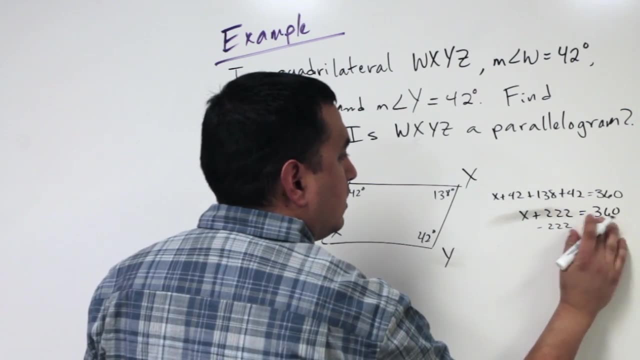 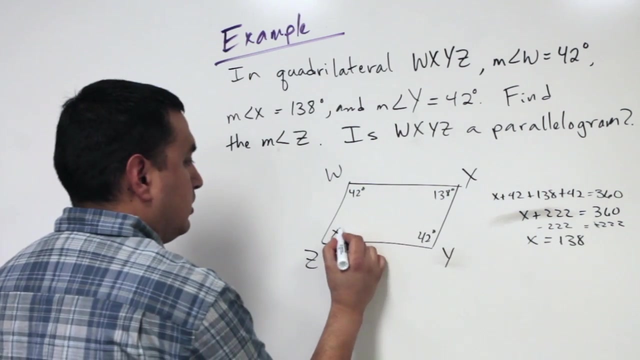 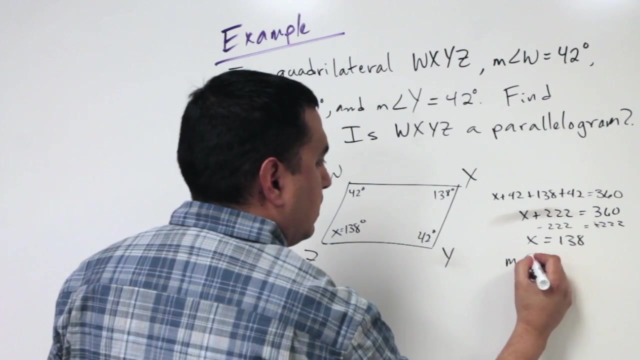 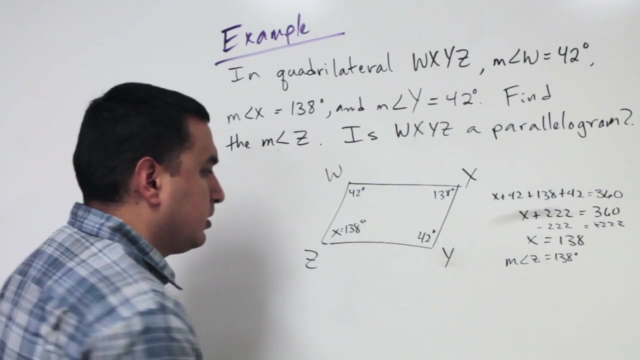 let's write it the other way: X plus 222 is equal to 360. if I subtract the 222, I get that X is 138. okay, so the measure of angle Z is 138 degrees, okay. and then to answer this question: is W, X, Y, Z a parallelogram? 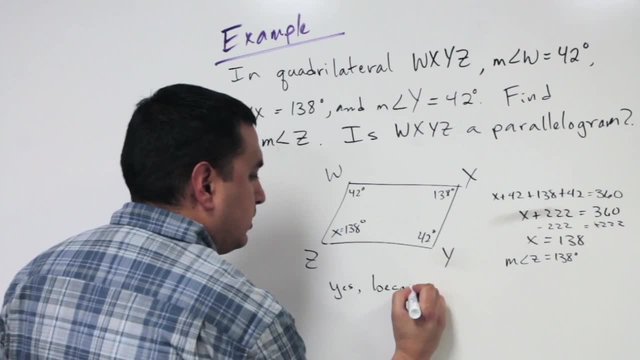 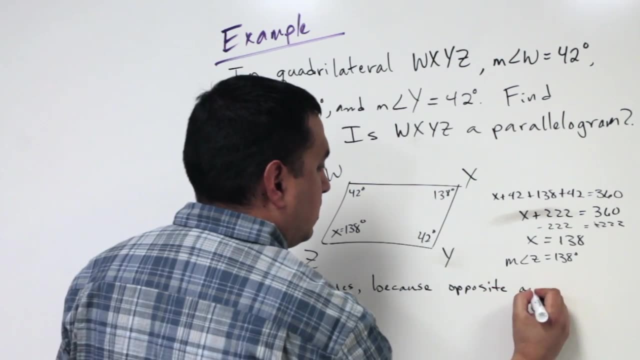 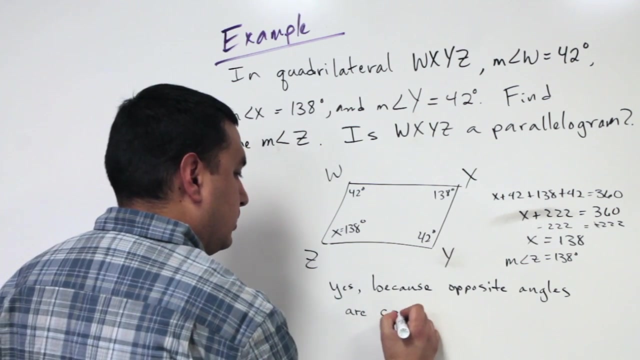 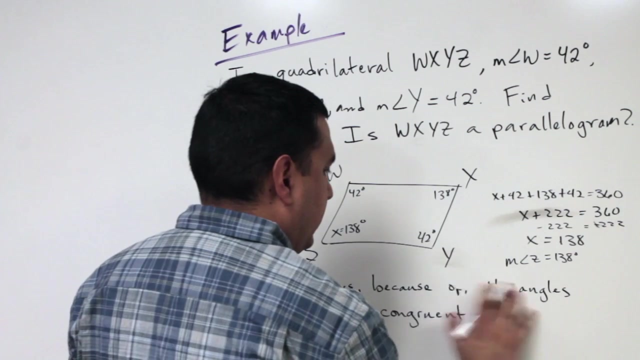 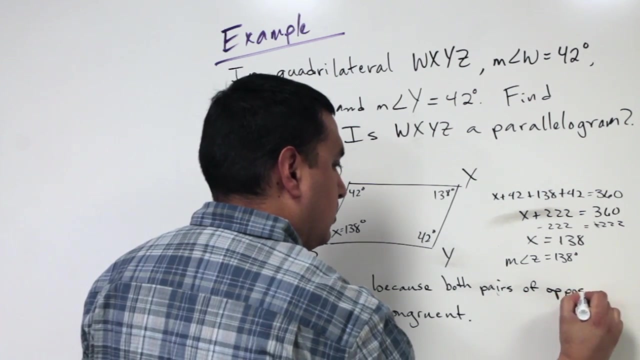 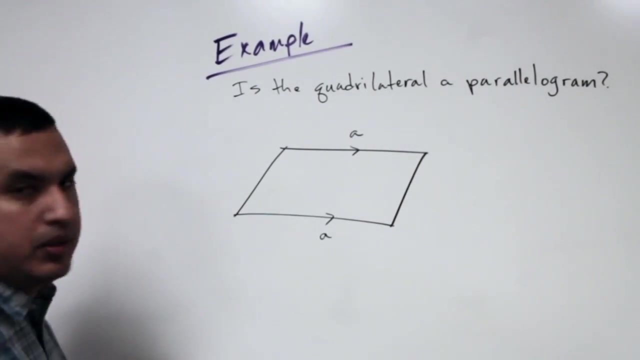 my answer would be yes, because I have opposite angles are congruent, and I guess I should say both pairs of opposite angles. yes, because both pairs of opposite angles are congruent. alright, so here's another example, and again we want to show if the quadrilateral, we want to explain, if this quadrilateral 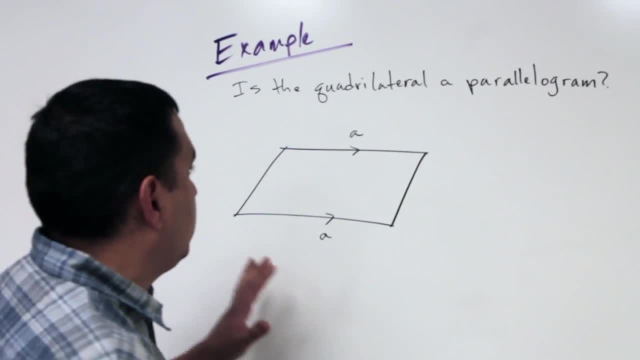 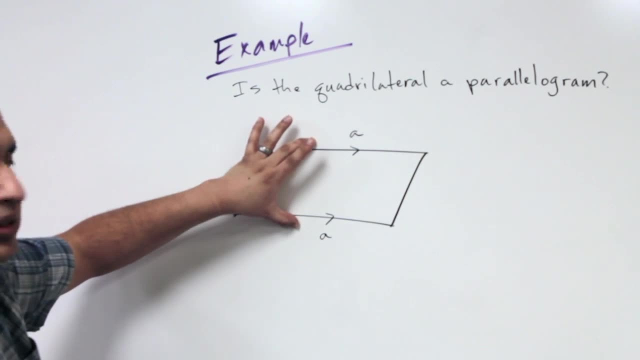 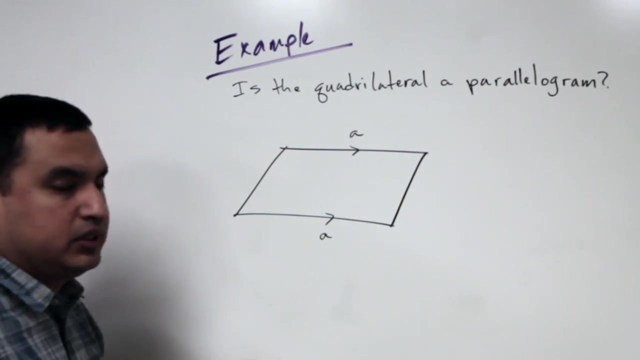 is a parallelogram. okay, this one. the answer is yes, and the reason for that is because I have a pair of parallel sides and those two sides are congruent. they both have this variable A. I don't know what they are, what that variable stands for. 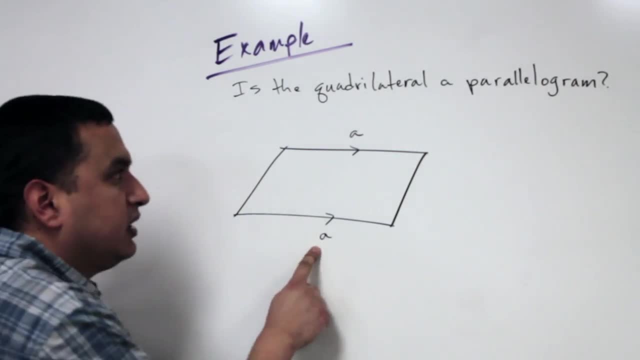 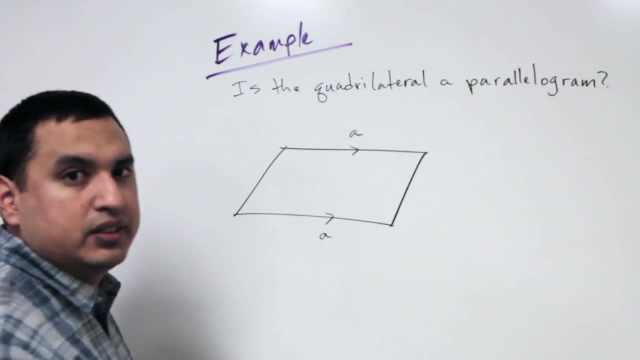 as far as a number, but if this side is some length A, this side up here also has to be some length A, so they're congruent and parallel. so I know, yes, this is a parallelogram. alright, here's a different type of problem. we're still trying to show that this quadrilateral is a parallelogram. 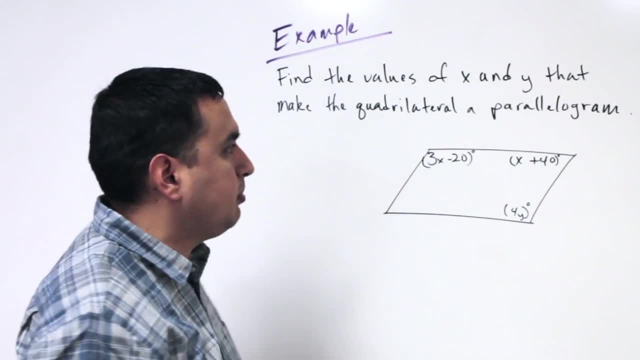 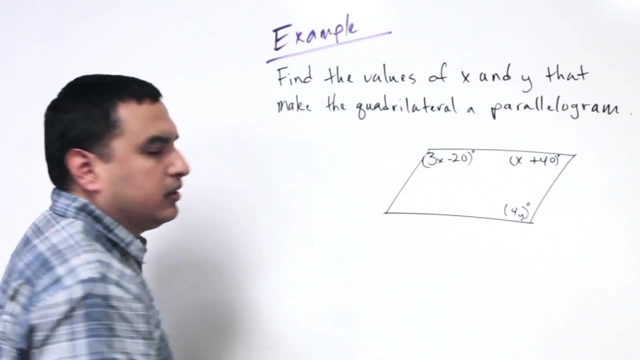 but they want us to think that, but they want us to figure out the values. that would make it a parallelogram. so I have this 3x minus 20, x plus 40 and 4y here. so if it is a parallelogram, 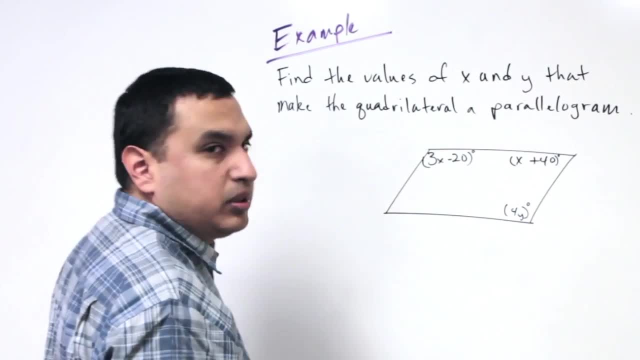 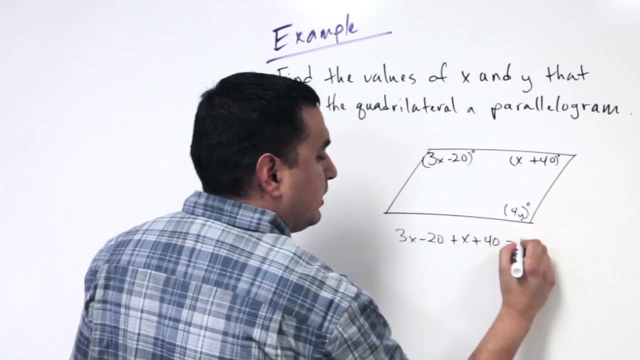 I know that consecutive angles are supplementary. so to solve for x I would have to do 3x minus 20, plus x plus 40 and set that equal to 180 degrees. if I combine like terms it gives me 4x minus or plus 20. 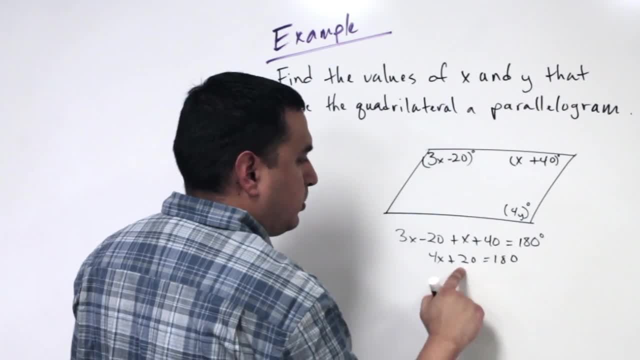 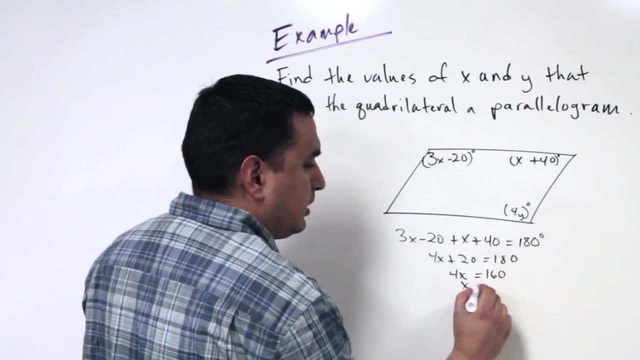 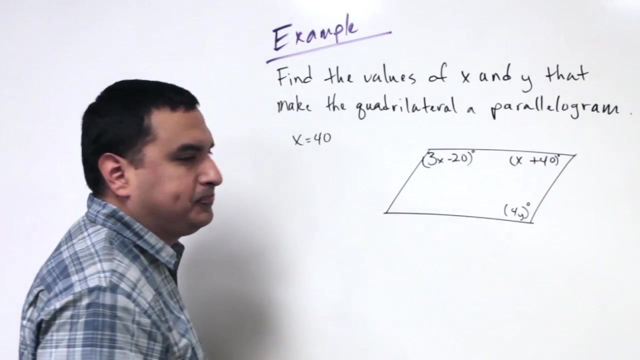 is equal to 180. subtract 20 gives me 4x equals 160, and then if I divide by 4, that tells me that x is 40. ok, so that's ok. the other part of now we can solve for y, the other side over here. 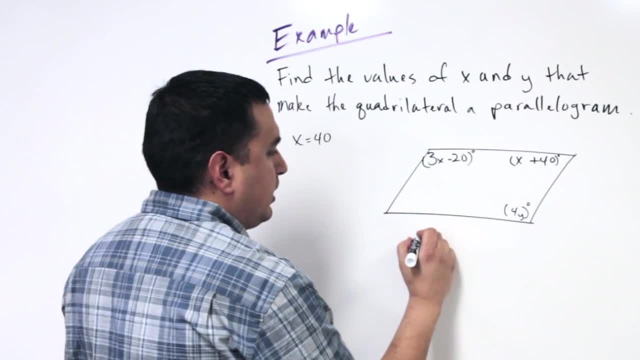 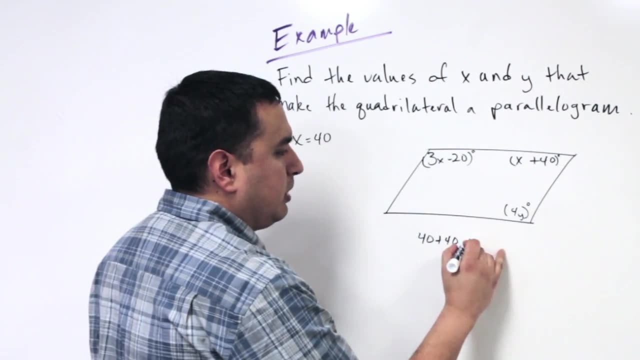 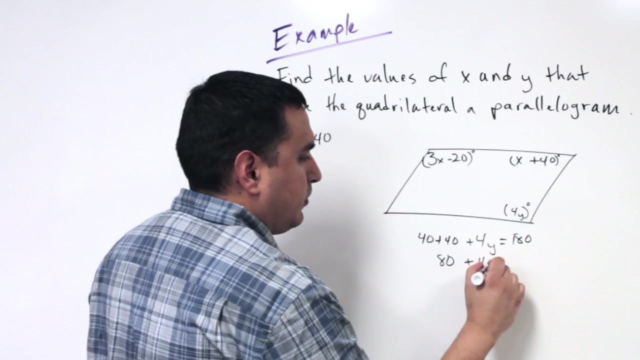 these are consecutive, so that means I can do 40 plus 40. if I substitute my 40 for x, I know that 40 plus 40 plus 4y has to equal 180. ok, so this gives me 80 plus 4y equals 180. 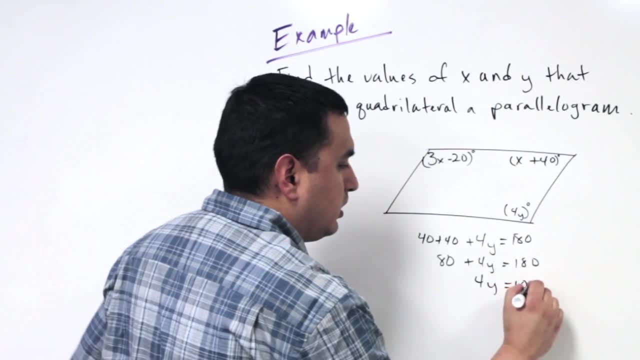 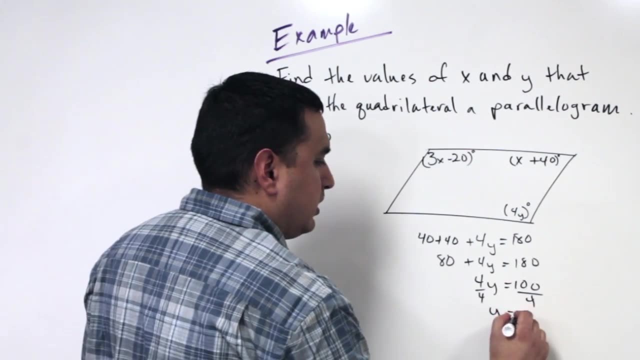 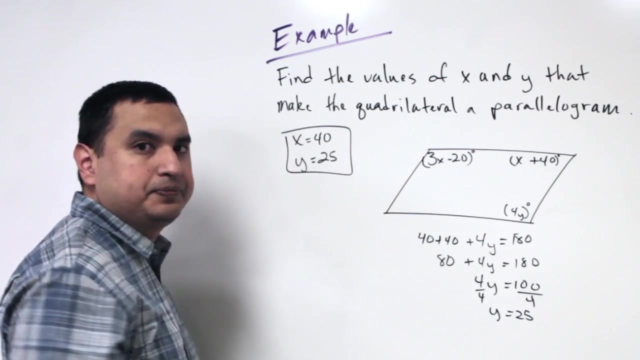 subtract 80 from both sides tells me that 4y is 100. and then if I divide by 4, that tells me that y is going to be 25. so for this problem, x is 40 and y is 25. ok on this example. 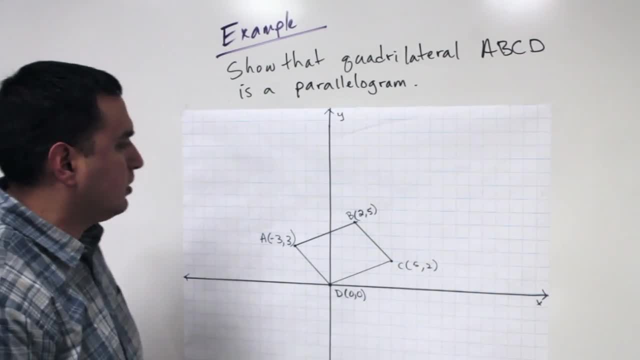 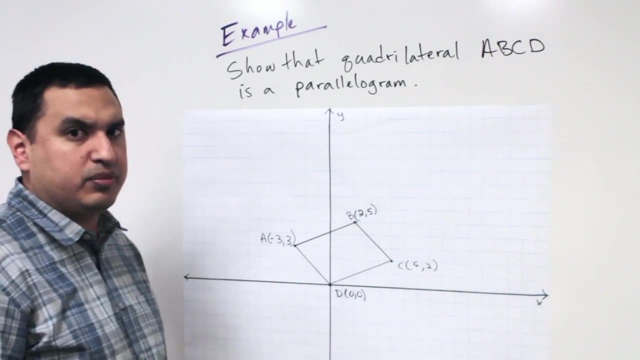 it wants us to show that the quadrilateral ABCD is a parallelogram. this time the quadrilateral is on the coordinate plane, so we're going to talk about it. we're still going to do the same things as far as different ways to prove that a quadrilateral is a parallelogram. 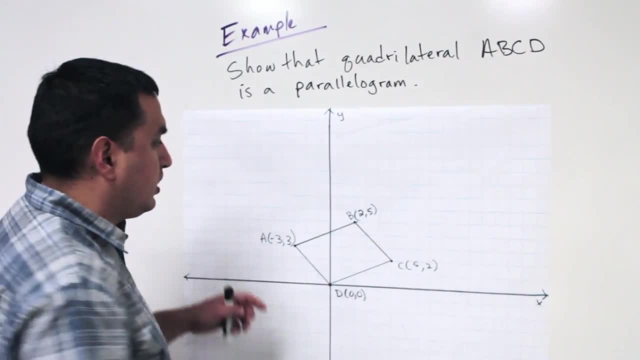 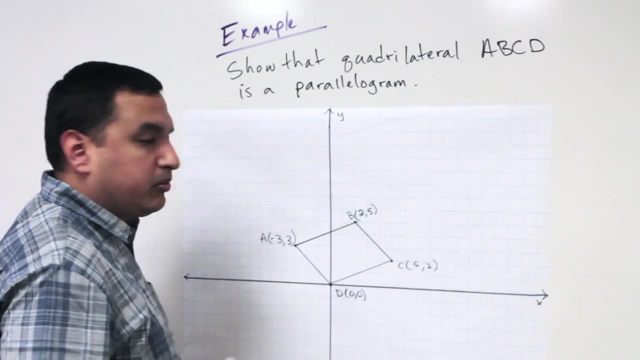 we're just putting it on a coordinate graph. I can do it two ways. I can show that the opposite sides are parallel for both. I can show these two sides are parallel and these two sides are parallel. that would be one way to show it if I can do that. 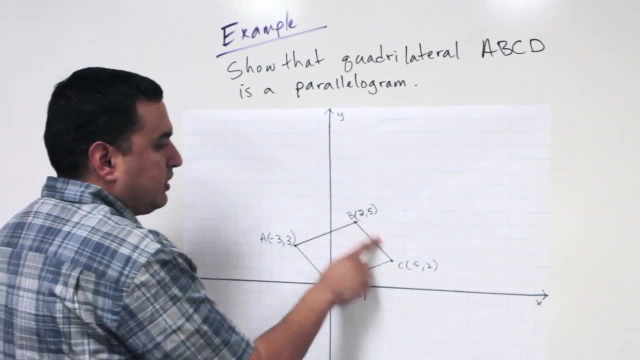 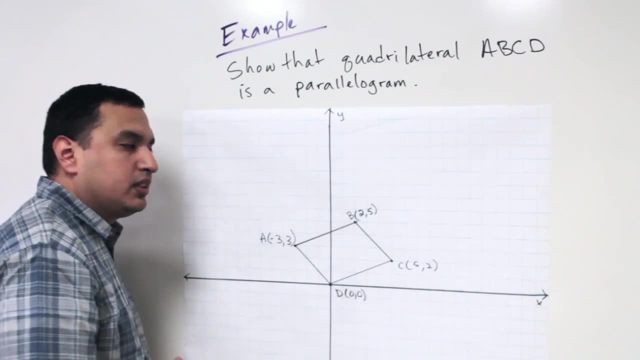 the other thing is I can just pick one side, like, say, if I looked at AD and BC and if I said, or if I showed that these two are parallel and congruent, then I know that I have a quadrilateral. ok, so let me zoom in a little bit. 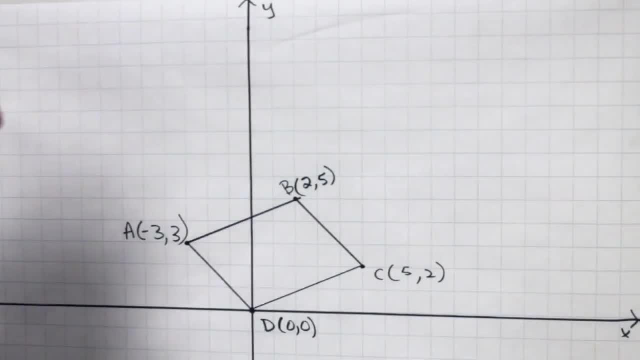 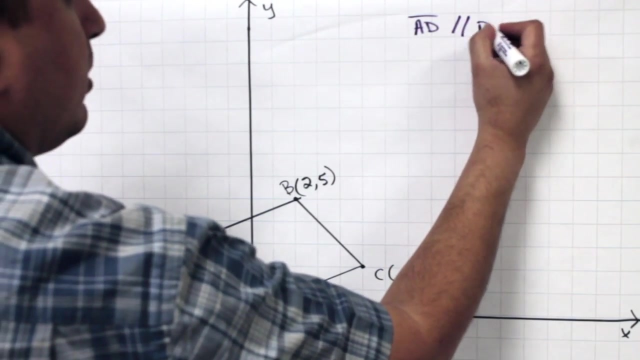 so that you can see what I'm doing a little better. ok, so let's start by showing that I'm going to pick AD and BC, and so I'm going to show. I'm going to look at this, I'm going to decide whether AD is parallel to BC. 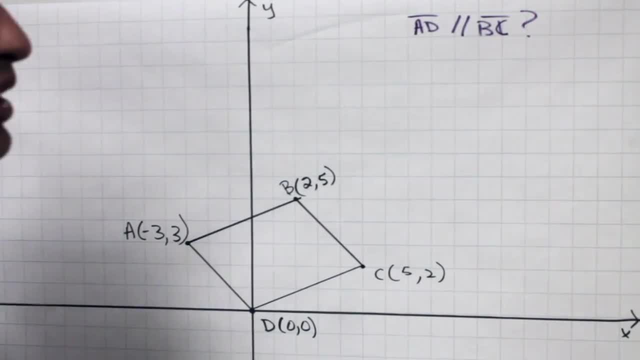 ok, so I'm going to. is that true or not? first thing I need to do for that is to look at the slopes. that's how I determine if they're parallel. so what I'm going to do for that is: I'm going to look at rise over run. 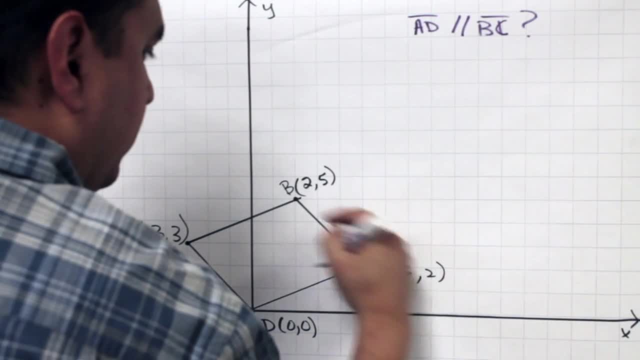 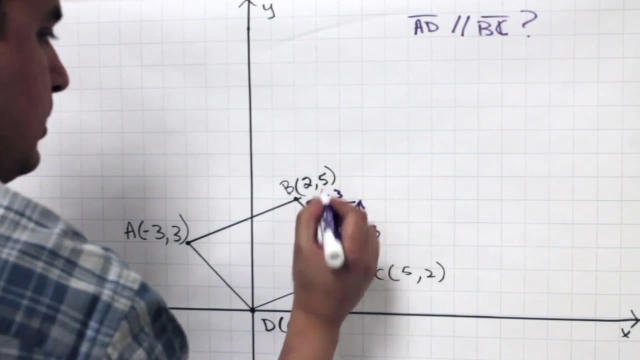 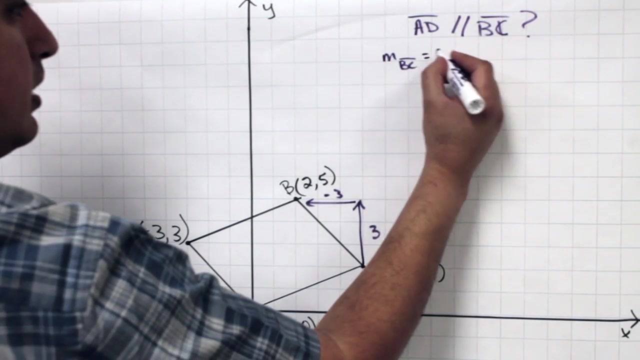 so if I'm looking at the slope of C to B or if I'm going from C to B, I go up 3 and left 3, so that's minus 3. so the slope of BC or CB is going to be negative 3 over 3. 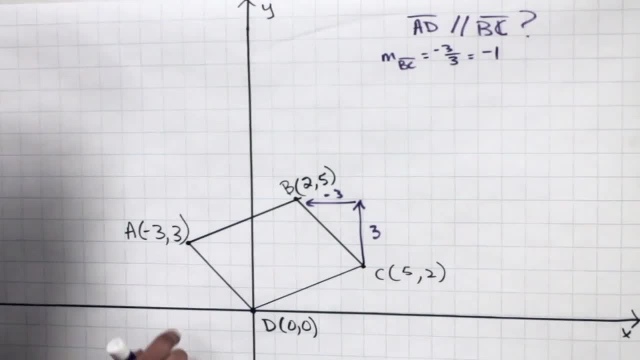 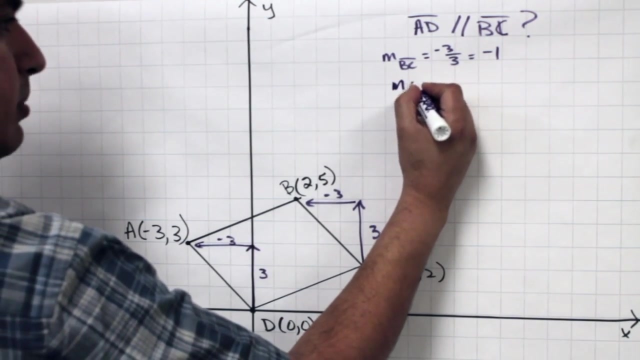 which is just negative 1. ok. now I want to do the same thing for AD. so if I'm looking at that, I'm going to go up 3 and I go back 3, so that's negative 3. ok. so the slope of segment AD. 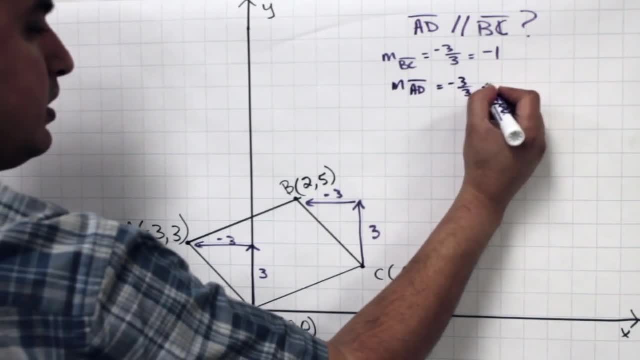 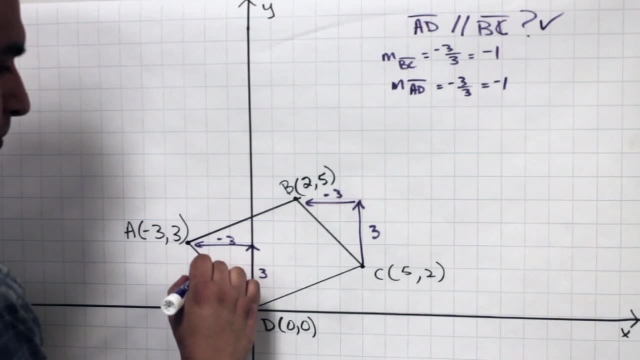 is also negative 3 over 3, which is negative 1. so, yes, I know that these two sides are parallel. ok, now I have to show if they are congruent. now, to do that, we're going to have to look at the distance formula. ok, so I need to find the length. 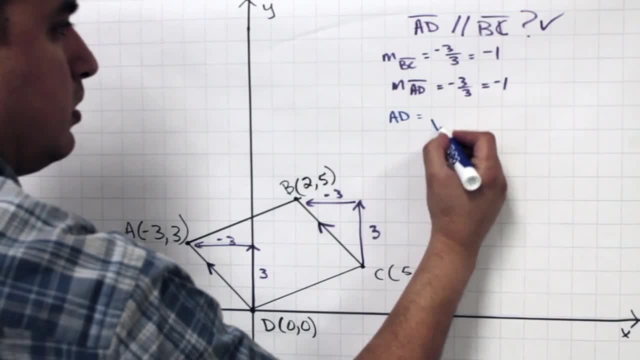 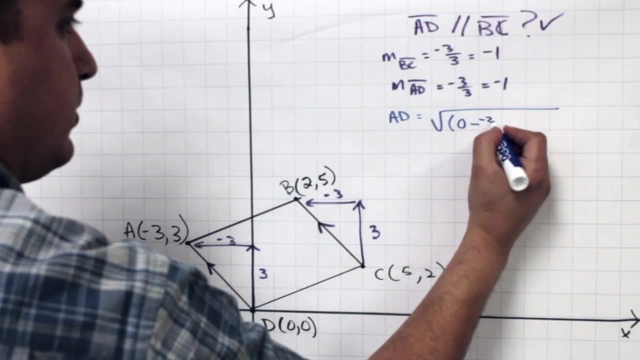 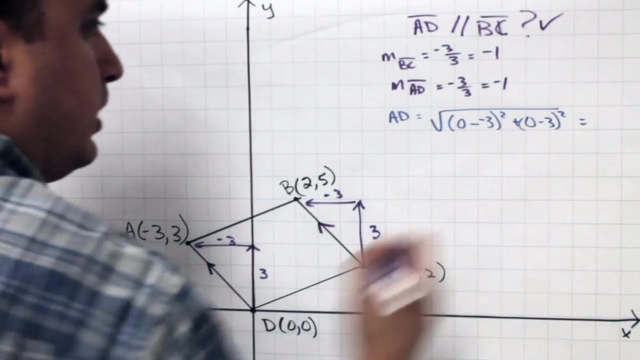 of AD. so we're going to do our x2 minus x1. so it's going to be 0 minus a negative 3 squared, plus 0 minus 3 squared. ok, now what that comes out to be: that's going to be 3 squared. 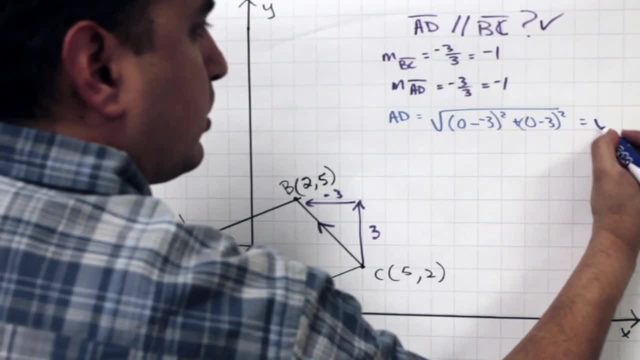 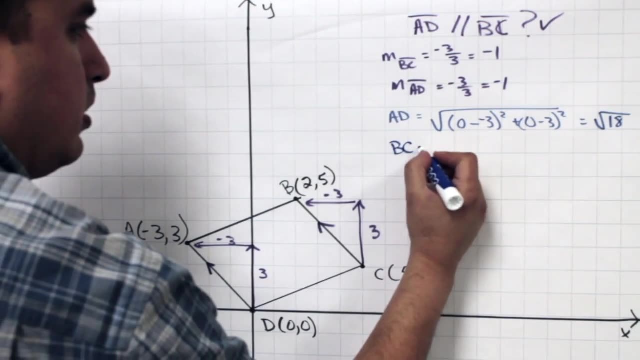 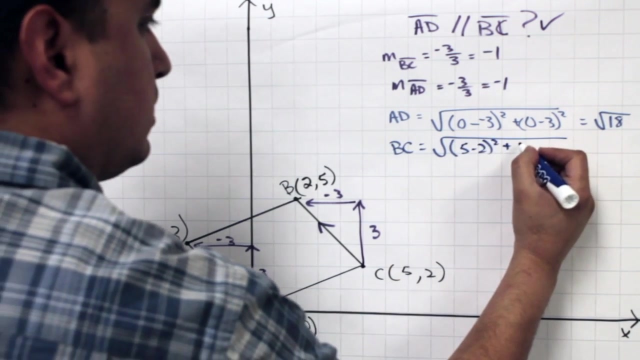 and negative 3 squared, so that's 9 plus 9. so this comes out to the square root of 18. ok, now we're going to do the same thing with BC. alright, so I got 5 minus 2 squared, plus 2 minus 5 squared. 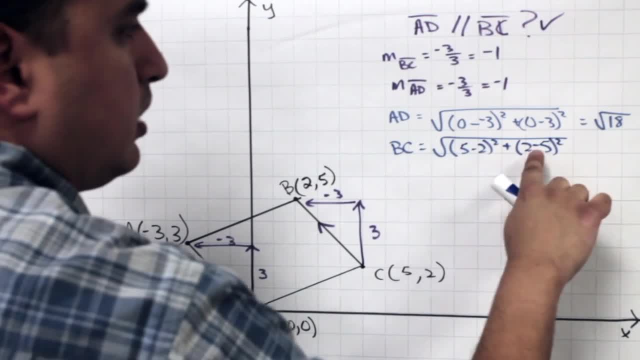 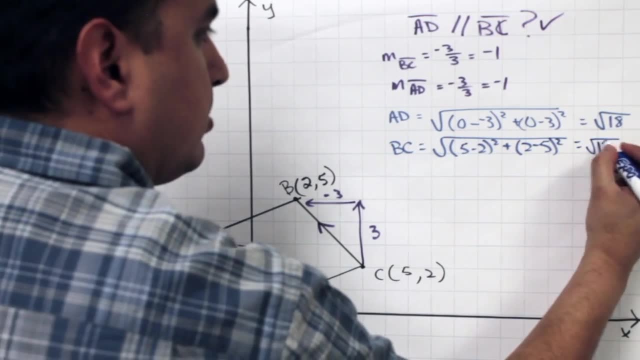 ok. 5 minus 2 is 3, so that's 3 squared. 2 minus 5 is negative 3, which is negative, 3 squared. ok, so both of those. if I put those in, that comes out to the square root of 18, ok, and which means that: 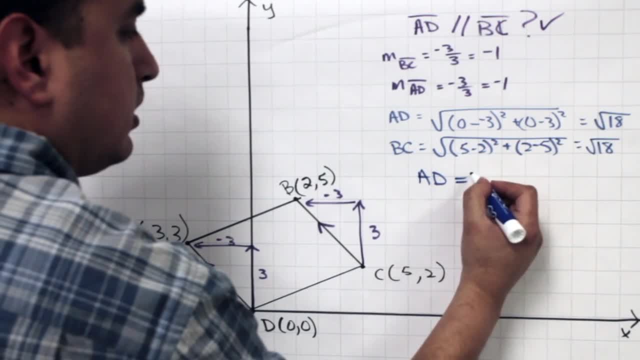 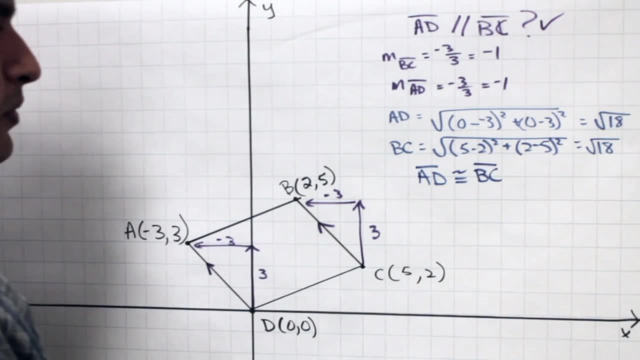 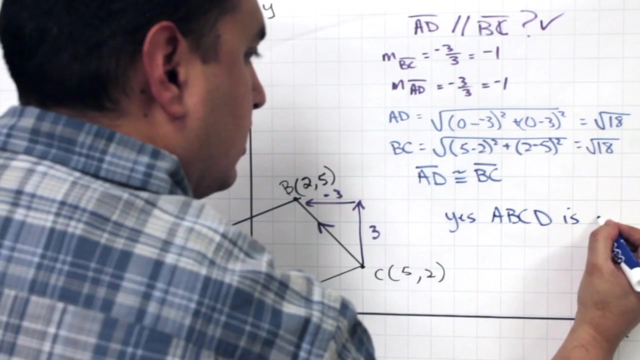 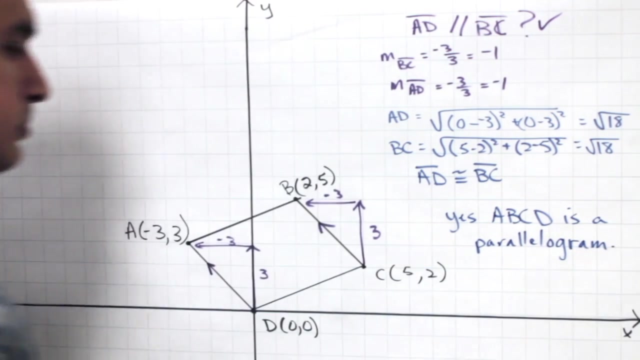 AD. the length of AD of segment AD is congruent to segment BC. so then I would say yes, ABCD is a parallelogram. 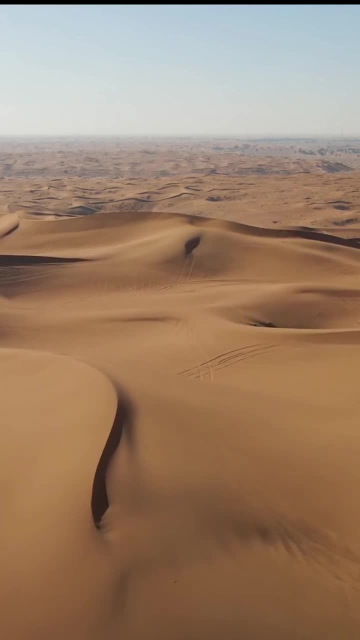 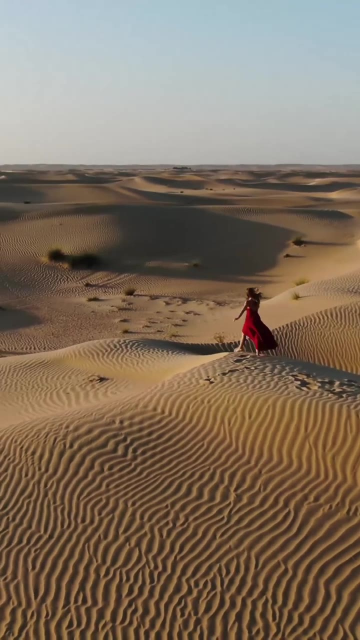 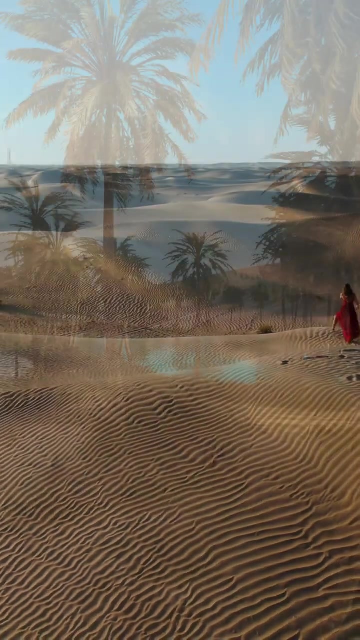 Welcome to Saudi Arabia, a land of contrasts where the climate is dry and temperatures soar high. The desert dominates this region and its vast expanse of red sand has witnessed hundreds of years of history, But in recent times, Saudi Arabia has been undergoing a remarkable transformation. 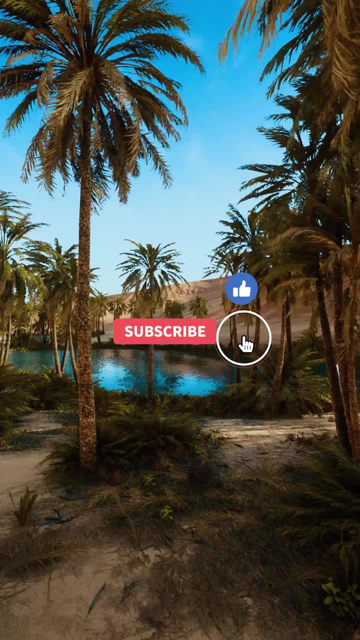 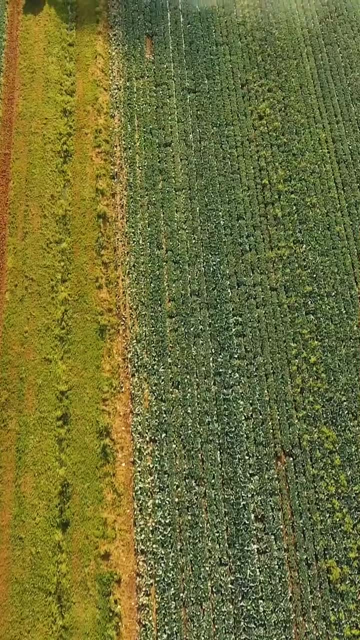 What was once a barren desert is now turning into a lush landscape of greenery and fields of flowers. But how is this possible in a region with such a harsh climate? Through innovative technologies and sustainable practices, Saudi Arabia has been able to turn the impossible into. a reality. The country is now home to some of the world's largest solar plants and has invested heavily in green technologies to create a more sustainable future. As a result, the desert of Saudi Arabia is no longer just a barren wasteland, but a thriving ecosystem with a bright and 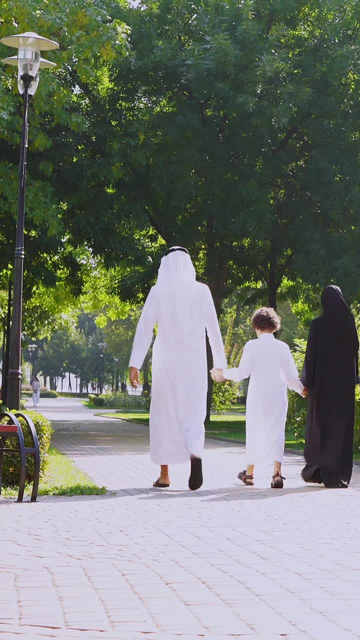 promising future. So come and witness the beauty and marvels of Saudi Arabia, where ancient history meets modern sustainability. 6. Saudi Arabia From the 27th century to the E hj Il 17th century. 3. Saudi Arabia From the 17th century to the 18th century. 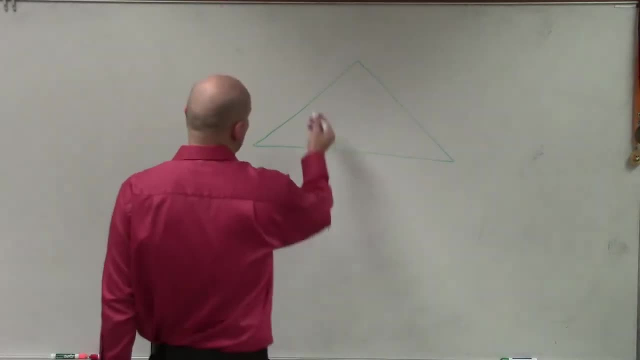 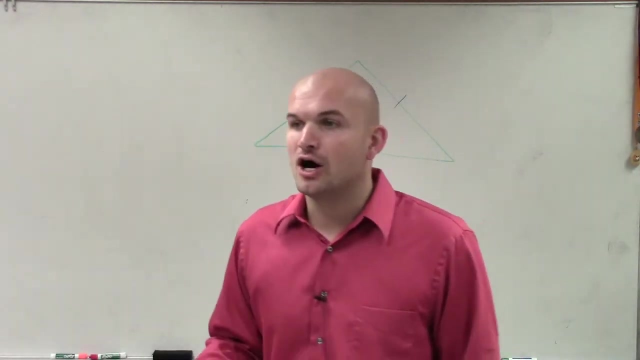 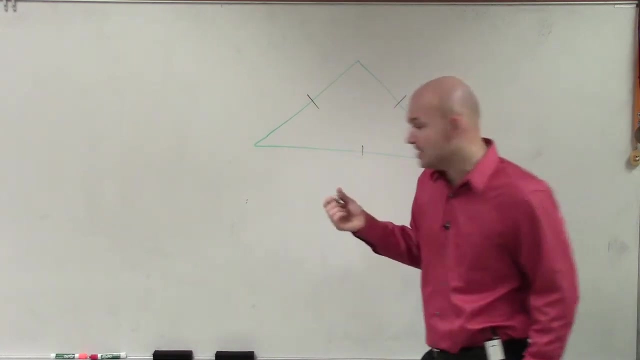 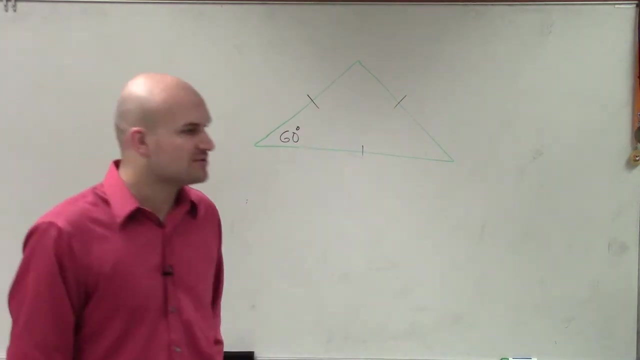 Okay. so in this example, question number five, they tell us that we have an equilateral triangle, meaning that each of every, all the measures of all the sides are equal in measure. I don't know if that made sense, but every side is equal in measure. Then they also said: find our remaining angles, which I didn't label this, but they gave us I know one angle which was 60 degrees. Now they said: you know pretty much to find the rest of the measures. Now one thing: we